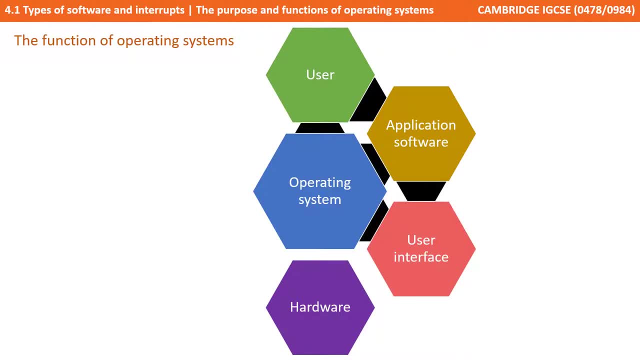 The application software will have a user and the operating system is providing a platform for those applications to run, and it's also providing its own user interface experience. in addition to the application software, There are also a number of utility programs, some of which are built into the operating system. 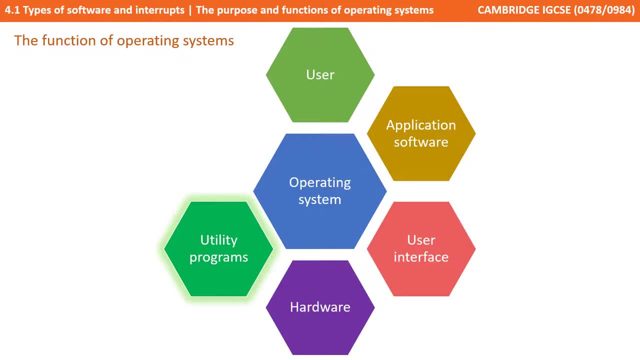 that help to maintain the computer. Some typical examples might be encryption software, compression software and defragmentation software. Loading the various programs into memory so they can be executed, and managing the data that those programs acquire is not a trivial task. So a very important part of your operating system is memory management. 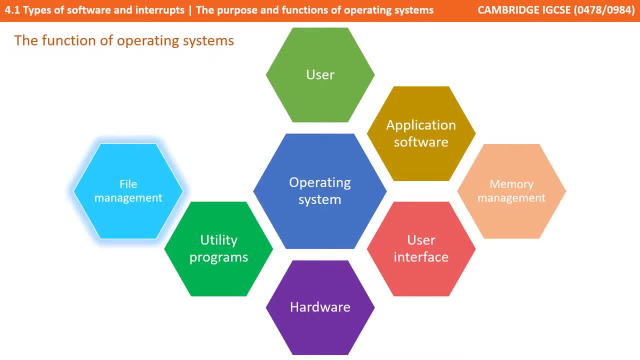 The user will also want to save what's in the memory from time to time so they don't lose their work when the power's switched off. So the operating system also has to manage the file store. It has to make decisions about where files are going to be stored and where they're going to be. 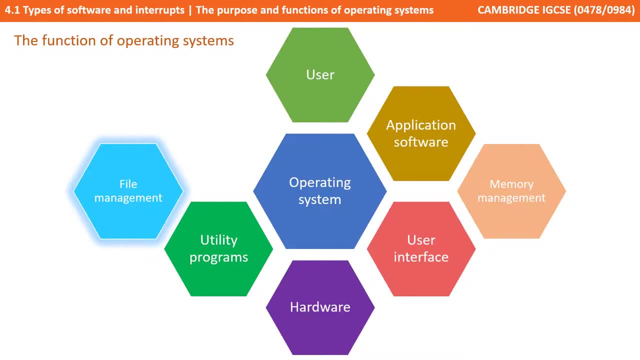 loaded from again. The operating system also has to manage the file store. It has to make decisions about where files are going to be stored and where they're going to be loaded from again. The large array of additional peripheral hardware connected to computers are also going to operate in a very specific way. 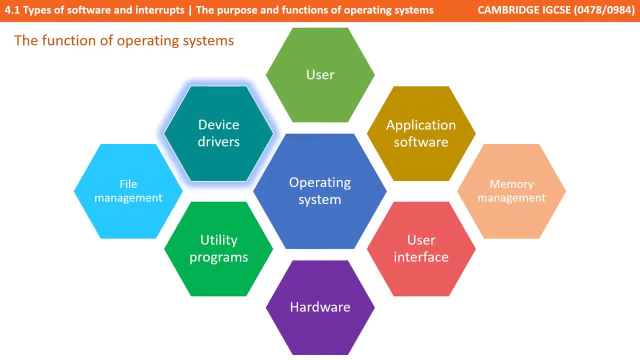 And therefore they need some device drivers in order to translate operating system instructions into something that the hardware is actually going to understand. The operating system is also responsible for handling and dealing with what are known as interrupts. This is when any device requires a device to run. 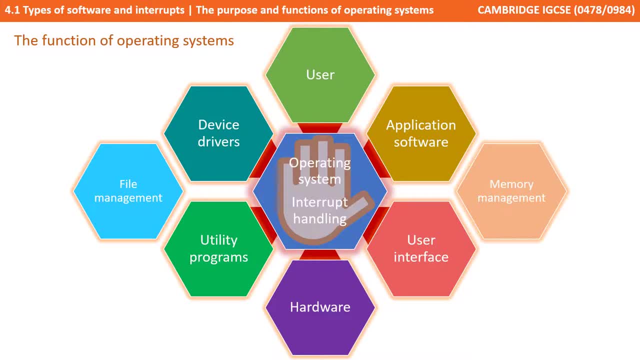 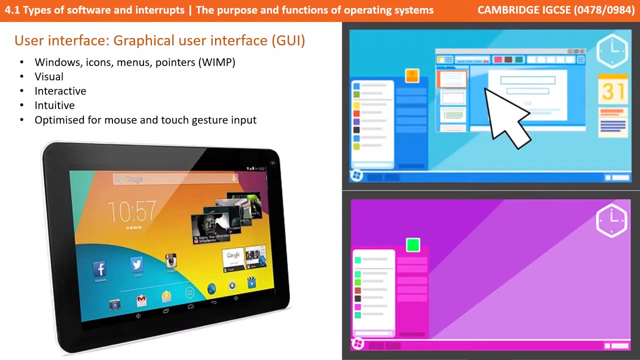 the attention of the processor. This could be quite dramatic, as in a power failure or something that seems quite trivial like a user pressing a key on a keyboard. We look at interrupts in more detail in a later video. The user interface, which is a catch-all umbrella term. 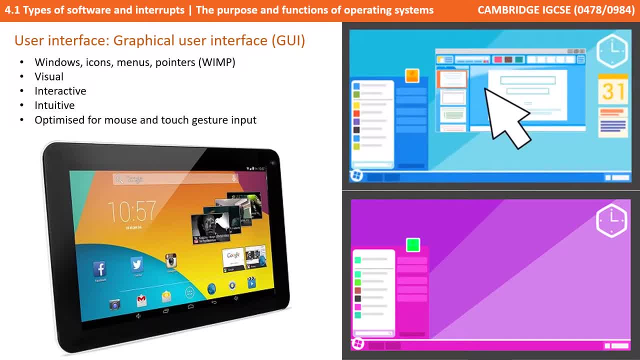 for the way in which you interact with a computer as a human being. There are a number of ways of providing that interaction by an operating system, And one of the most common and familiar to you is what's known as the graphical user interface or GUI. 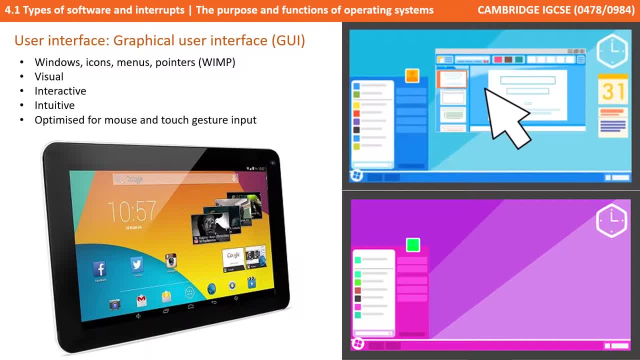 So here we've got Windows, we've got icons, we've got menus and we've got the pointer, And this is often known as a WIMP interface: Windows, icons, menus and pointers. It's a very visual interface and it's very interactive. 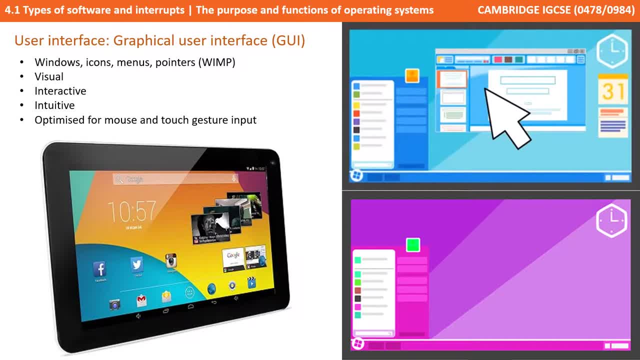 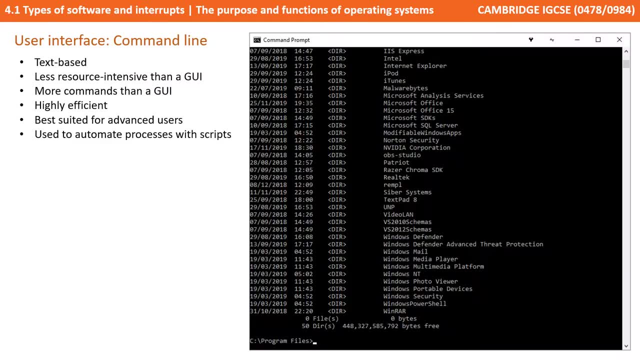 It's quite intuitive to use, so it's ideal for beginners And it's optimized for the mouse and touch gestures and gesture input. The opposite of a graphical user interface is a command line interface. It's very text-heavy but it's less resource-heavy. 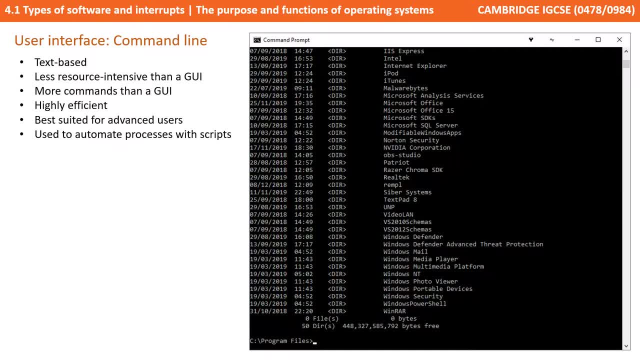 compared to a GUI, It's very slim-lined and efficient. It tends to have more commands than a graphical user interface. It's best suited for advanced users that want to accomplish tasks quickly. It's useful for automating process with scripts, And it's often the interface that's 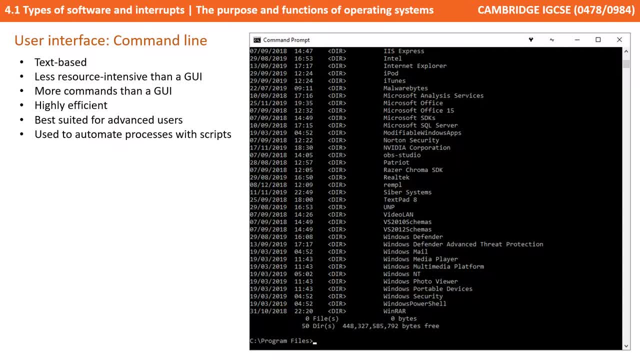 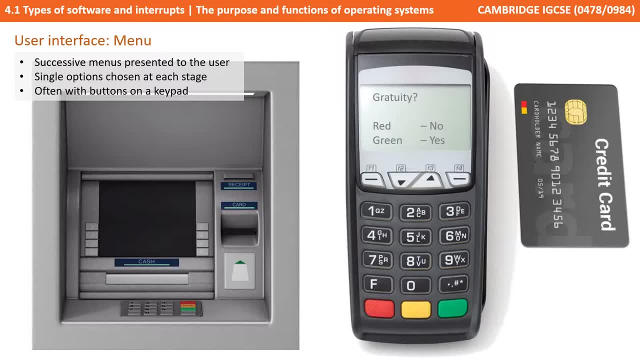 used if you want to do something quite technical with your computer. Another type is the menu-driven interface. This is the sort you're going to find at cache points and on chip and PIN devices. So here in this example, we see a chip and PIN device. 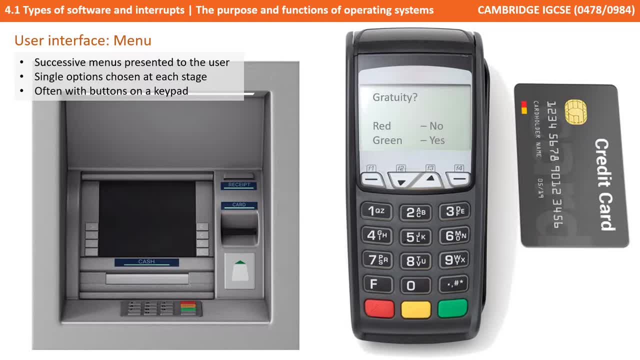 asking the user whether they want to give a gratuity, a tip, And the user is going to choose yes or no depending on the buttons they press. So we have successive menus presented to the user with a single option chosen at each stage. 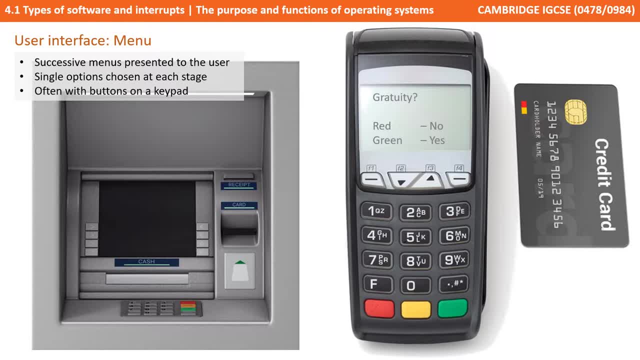 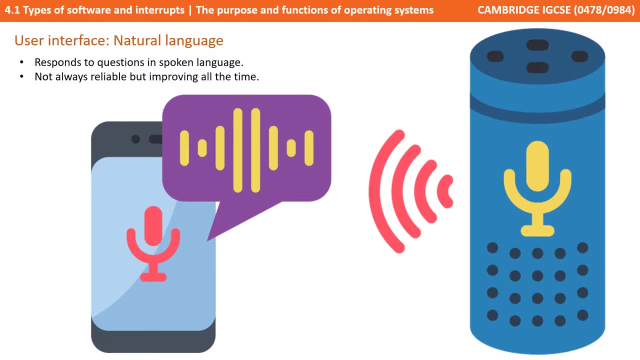 And you often interact with them via buttons on a keypad. A user interface that's gaining popularity today is the natural language interface, the idea that you can actually speak in your natural language into a computer system so it responds to question, for example, said in spoken English. 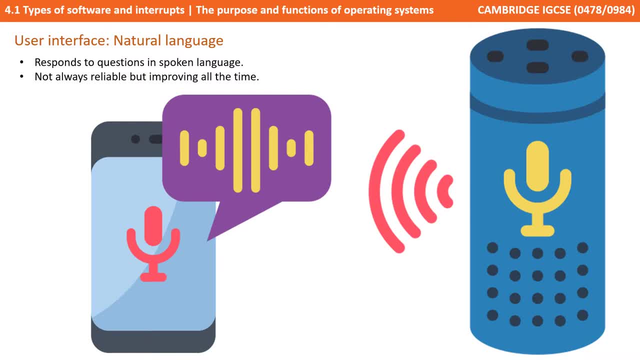 The historical problem with these interfaces is they're often not very reliable, but the technology is certainly gaining in pace and accuracy. Siri, Cortana, Hey, Google and Alexa are all examples of this, And it is pretty cool to be able to say to a device: hey Siri. 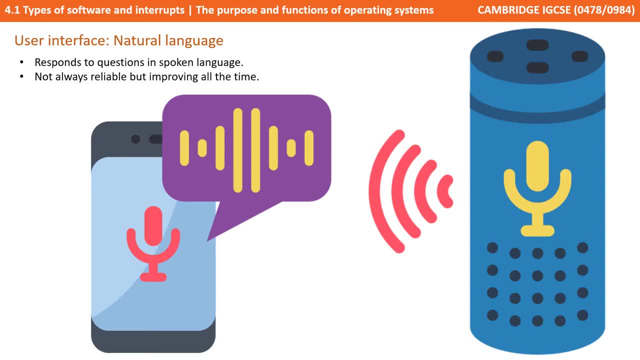 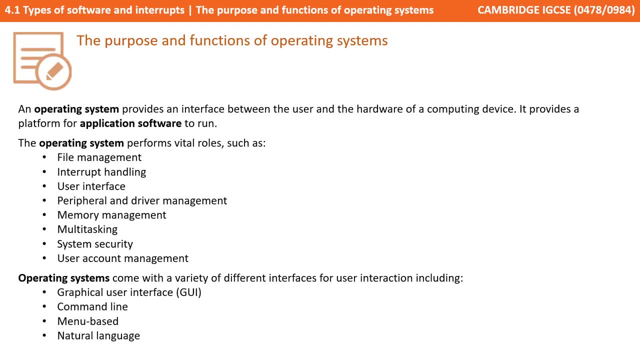 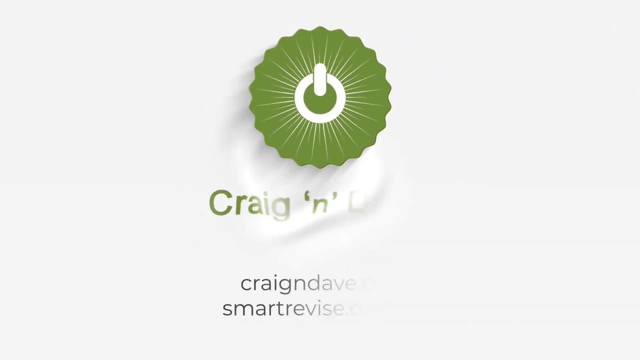 what's the weather today? Or Alexa, how many emails haven't I read? That's everything for this video. Here's a summary of what you've learned, So pause and take some notes. Thank you for watching.